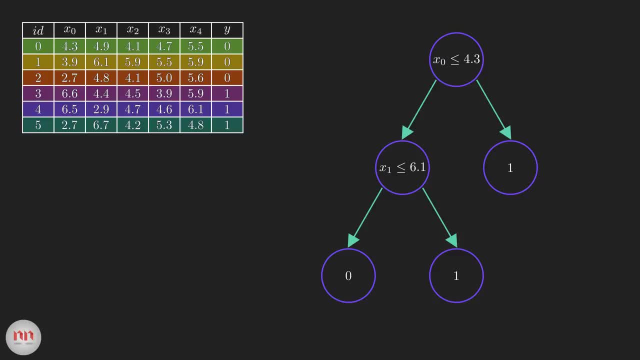 label is assigned to it. So what's the problem with decision trees? Let's change our training data slightly. Focus on the row with ID 1.. We are changing the x0 and x1 features. Now, if we train our tree on this modified dataset, we will get a completely 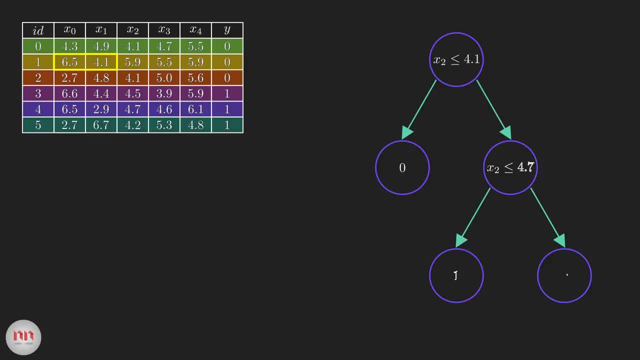 different tree. This shows us that decision trees are highly sensitive to the training data, which could result in high variance, So our model might fail to generalize. Here comes the random forest algorithm. It is a collection of multiple random decision trees and it's much less sensitive. 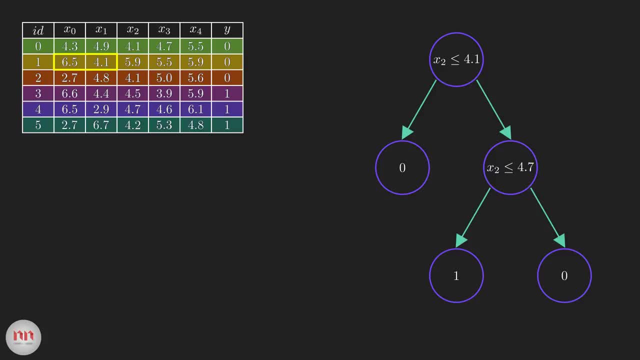 to the training data, You can guess that we use multiple trees, hence the name forest. But why is it called random? Keep this question in the back of your mind. You will get the answer by the end of this video. Let me show you the process of creating a random forest. 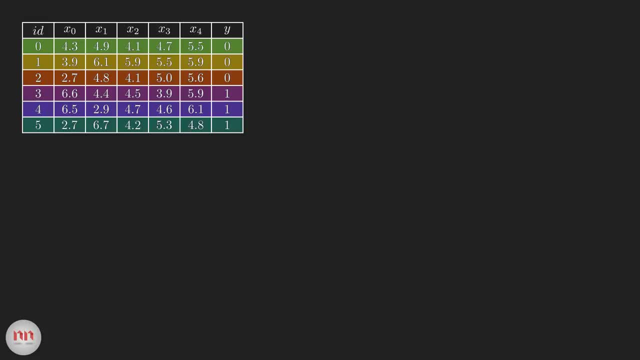 The first step is to build new datasets from our original data. To maintain simplicity, we will build only four. We are going to randomly select rows from the original data to build our new datasets, And every dataset will contain the same number of rows as the original one. 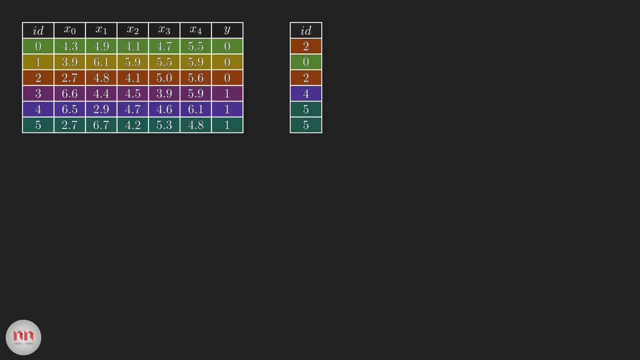 Here's the first dataset. Due to lack of space, I am writing only the row ids. Notice that row 2 and 5 came more than once. That's because we are performing random sampling with replacement. That means after selecting a row, we are putting it back into the data. 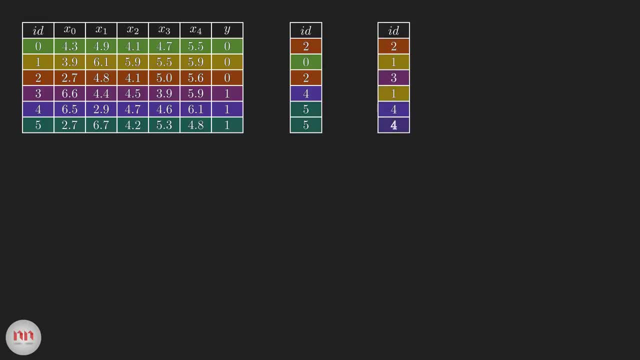 And here are the rest of the datasets. The process we just followed to create new data is called bootstrapping. Now we will train a decision tree on each of the bootstrap datasets independently. But here's a twist: We won't use every feature. 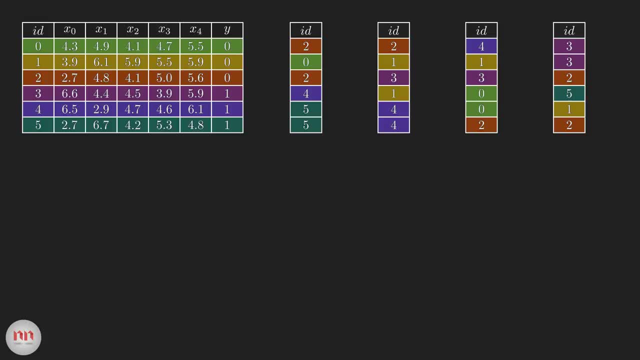 for training the trees. We will randomly select a subset of features for each tree and use only them for training. For example, in the first case, we will only use the features x0 and x1.. Similarly, we will only use the remaining trees Now that we have got the data and the feature subsets. 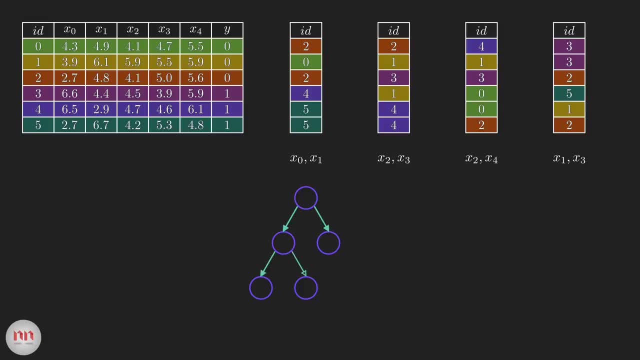 let's build the trees, Just see how different the trees look from each other. And this, my friend, is the random forest containing four trees. But how to make a prediction using this forest? Let's take a new data point. We will pass this data point through each tree, one by one. 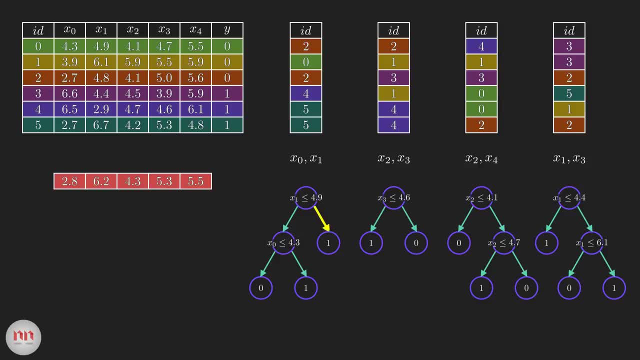 And note down the predictions So we can search and find all the previous predictions. And now let's check the prediction field So we can see that we have got the same number of predictions on each tree. Let's check out if the data was the ones which we didn't see at first. 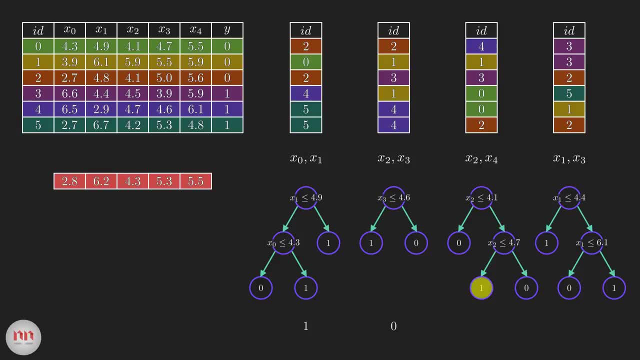 And yes, that's correct. And now that we have also found all the predictions from each tree, we can then update the data report. Now to tell you what we have done, We will need to take a new data point If we were to take the data from the tree on the first layer of the tree. 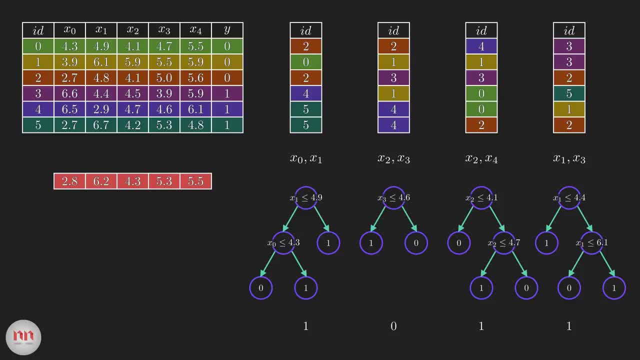 we will have to add the same data point to it along the secondary tree And then we will have to depend on the data point of each tree, which is the main tree, So we can click on the data point item majority voting. Clearly, 1 is the winner. Hence the prediction from our random forest is 1.. 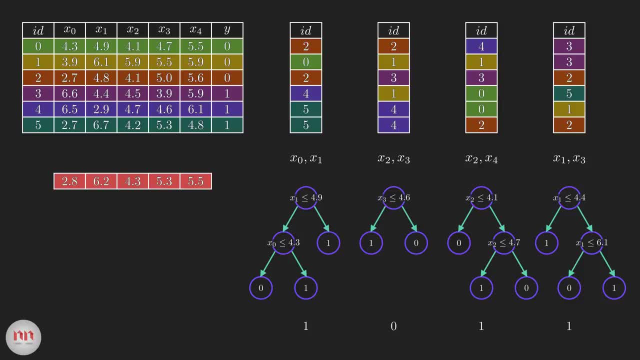 This process of combining results from multiple models is called aggregation. So in the random forest we first perform bootstrapping, then aggregation, And in the jargon it's called bagging. Okay, so that was how we build a random forest. Now I should discuss some of the very 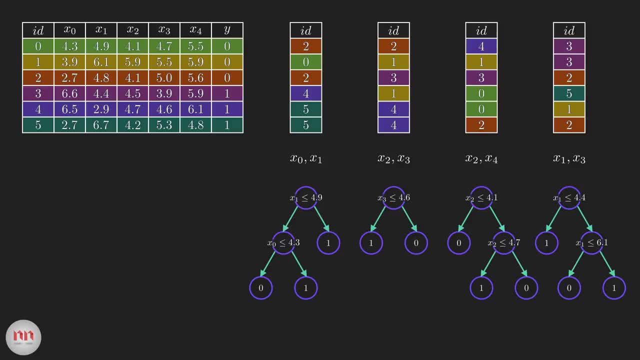 important points related to this algorithm. First, why it's called random? Because we have used two random processes: bootstrapping and random feature selection. But what is the motivation behind bootstrapping and feature selection? Well, bootstrapping ensures that we are not using the 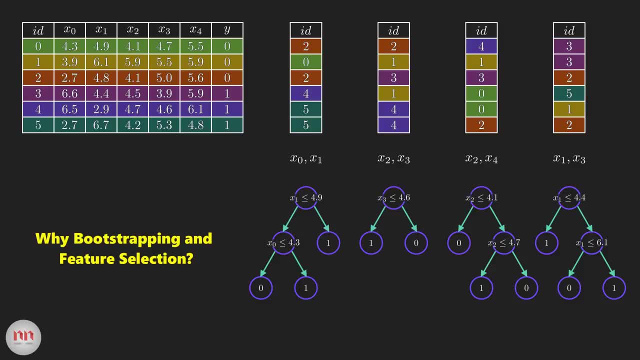 same data for every tree. So in a way it helps our model to be less sensitive to the original training data. So let's get started. Random feature selection helps to reduce the correlation between the trees. If you use every feature, then most of your trees will have the same decision nodes and they will act very